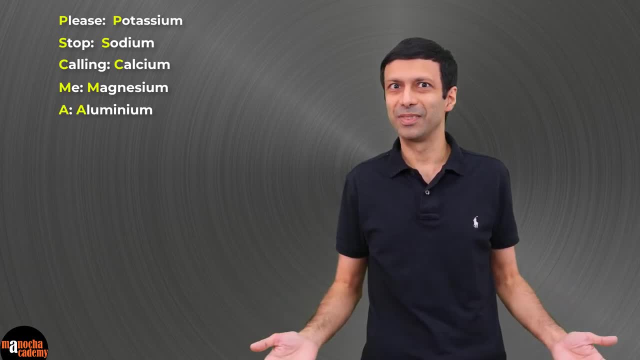 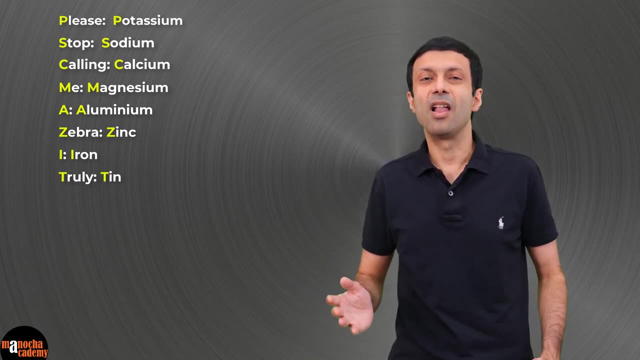 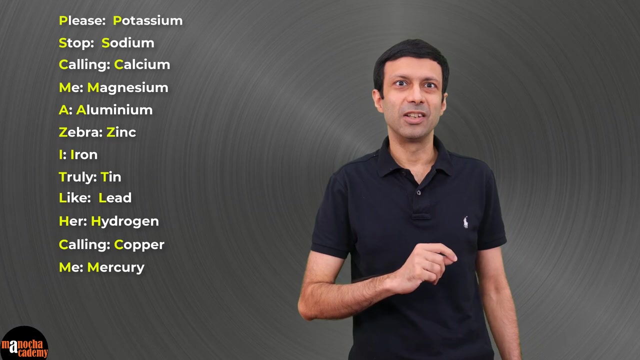 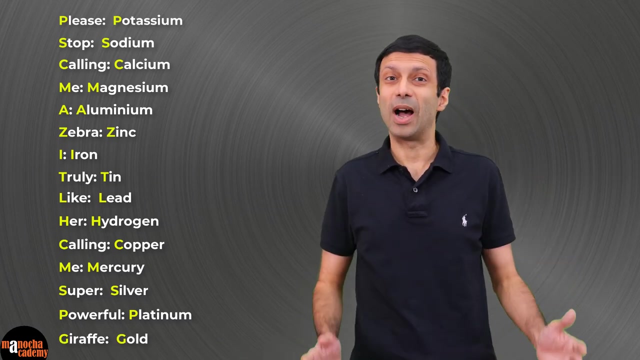 me for magnesium, a for aluminium, zebra for zinc, I for iron, truly for tin, light for lead, her for hydrogen calling for copper, me for mercury, super for silver, powerful for platinum and finally, giraffe for gold. So, as you can see, potassium is the most. 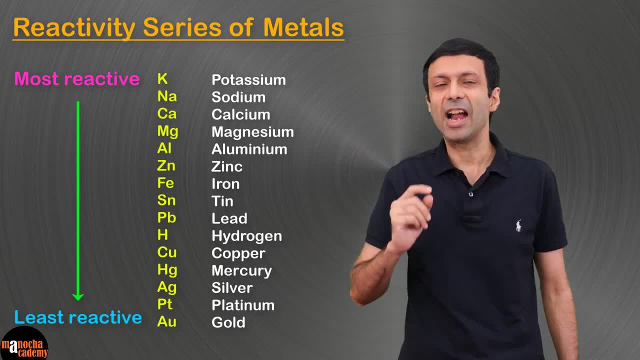 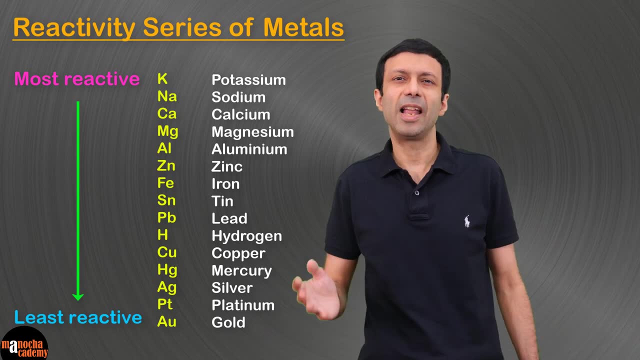 reactive metal, since it's at the top of the list, And gold is the least reactive, since it's at the bottom of the list. Now in some books you might see some variations, like platinum is written as least reactive metal instead of gold. But one interesting question is: what is Mr Hydrogen? 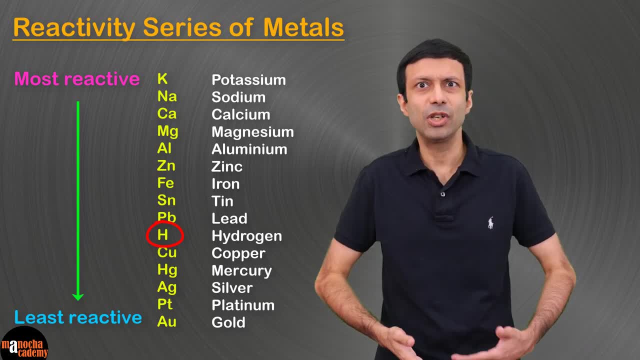 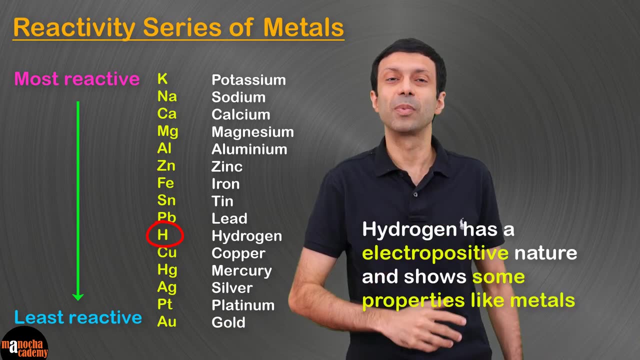 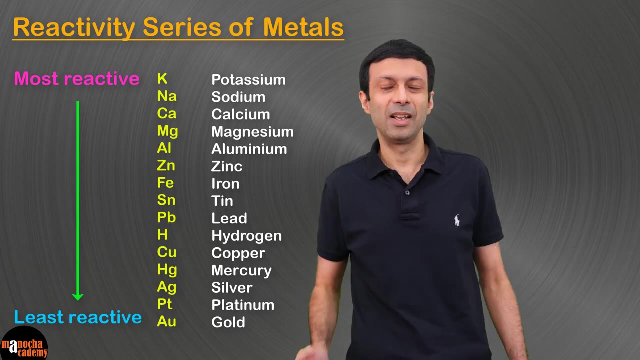 doing in this series of metals? Because hydrogen is a non-metal, it's a gas, But remember, it has an electropositive nature and shows some chemical properties like metals. That is why it is found in this reactivity series of metals. This reactivity series can be used to predict single displacement reactions, So it's. 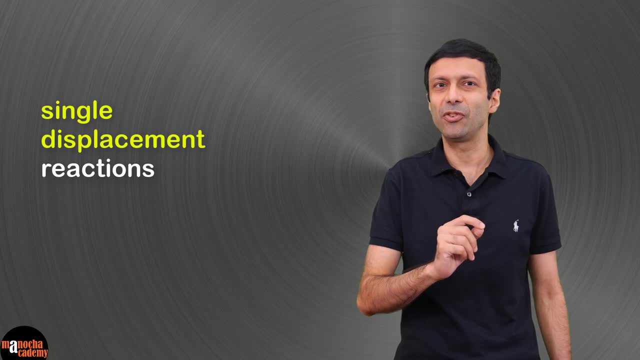 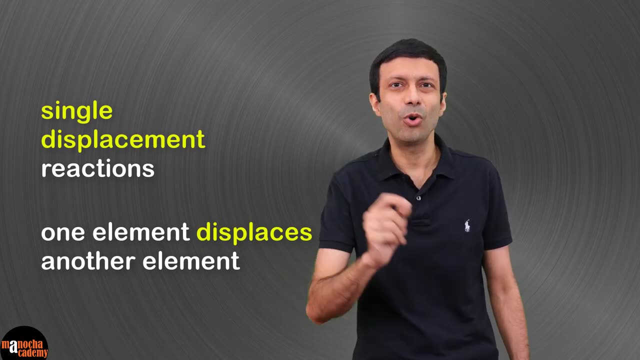 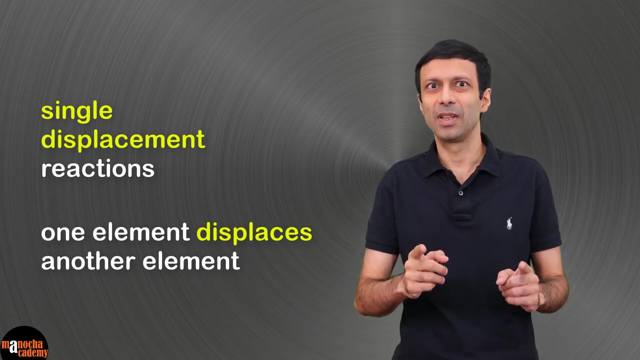 very useful. And remember, in a single displacement reaction, one element displaces another element. But remember that only a more reactive element can displace a less reactive element based on this reactivity series, For example, what will be the reaction when zinc reacts with dilute hydrochloric acid? 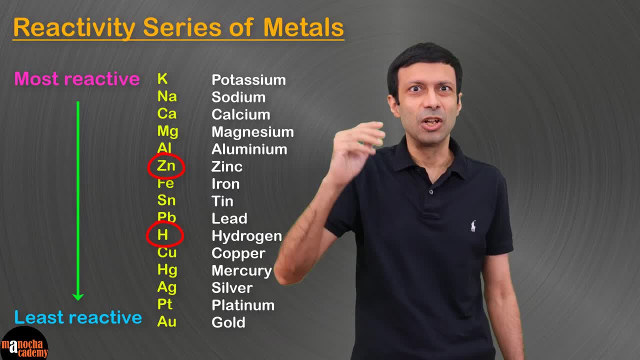 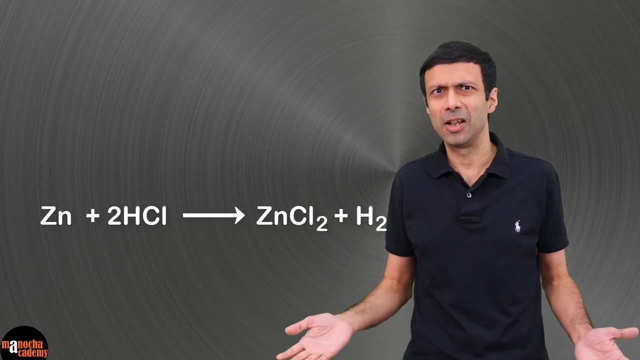 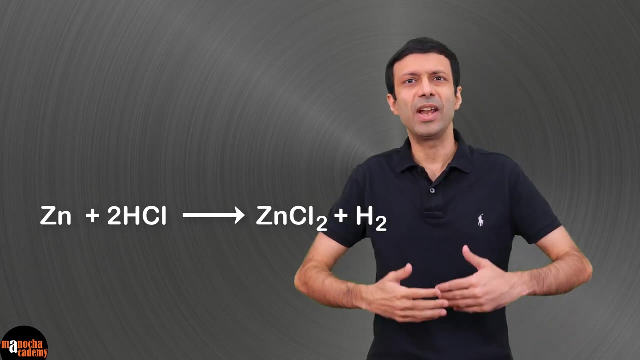 In the reactivity series, zinc is above hydrogen. So zinc will displace hydrogen in the acid and will get zinc chloride and hydrogen gas. Basically, zinc tells hydrogen to get out and displaces it. Now what will be the reaction if silver reacts with dilute hydrochloric acid? 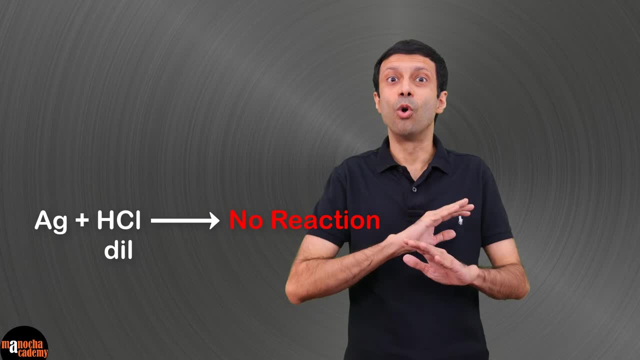 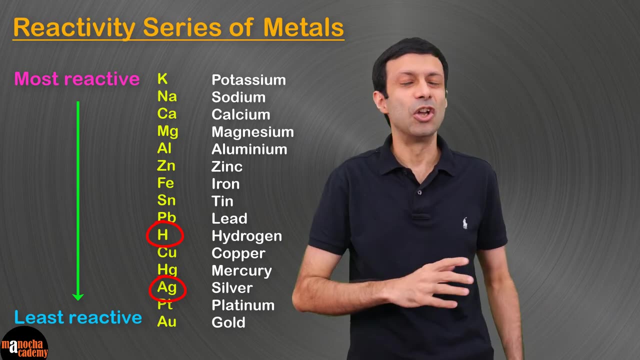 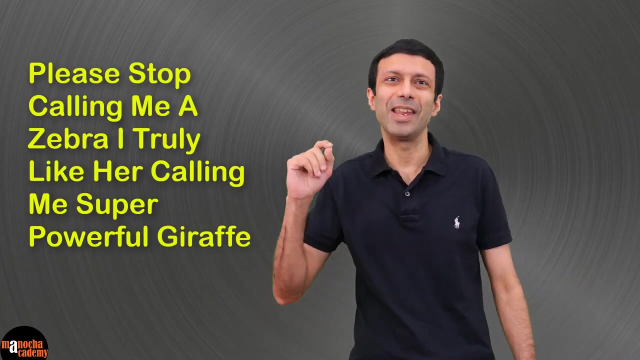 What do you guys think? The correct answer is no reaction. Why? Because silver is below hydrogen in the reactivity series, So silver cannot displace hydrogen. So hope you guys understood the concept of reactivity series and like this mnemonic that we learned today. If you guys know some other. 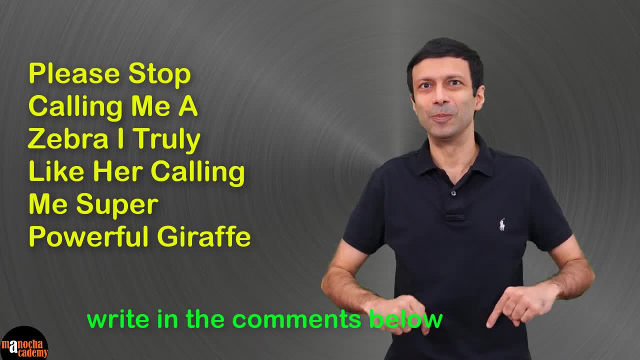 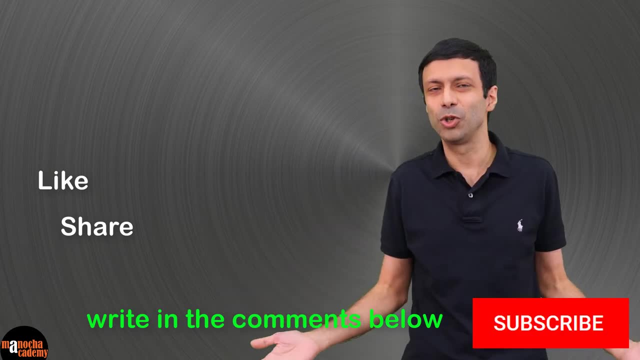 interesting mnemonic. do share it in the comments below. Thank you for watching. See you in the next video. Bye, And please hit the like button and share out this video with your friends. And if you still haven't subscribed to our YouTube channel, what are you waiting for?